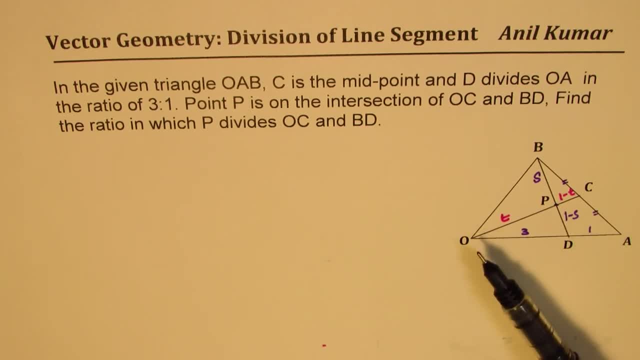 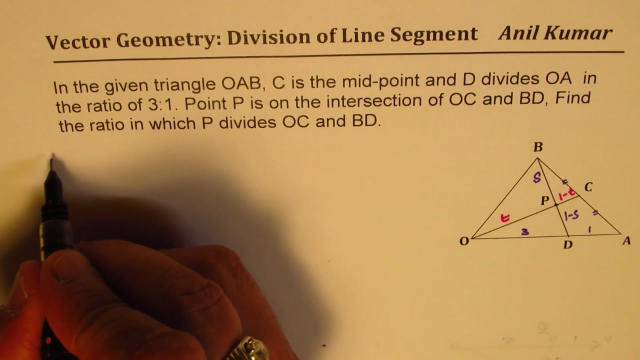 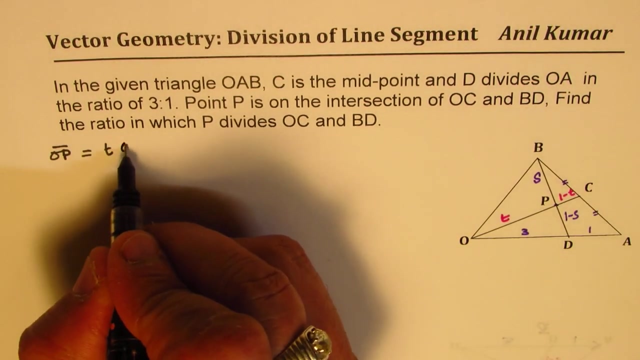 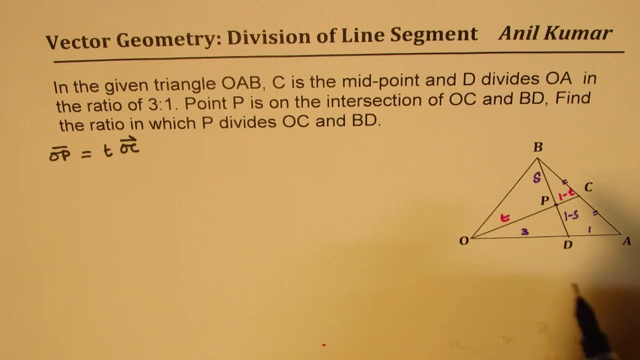 now, the idea here is to write OP in two different ways, involving both the parameters, and then we'll isolate them and figure them out. so let's first find what is OP from this direction. so we know OP can be written as T, the scalar multiple of OC. right now, what is OC? to get the value of OC, let us write down: 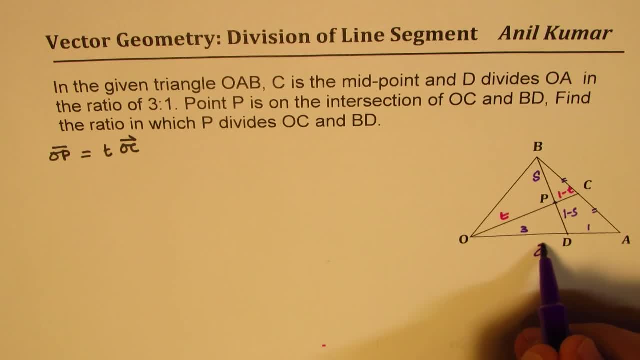 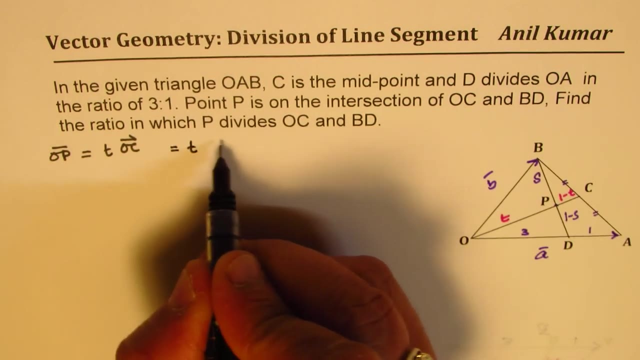 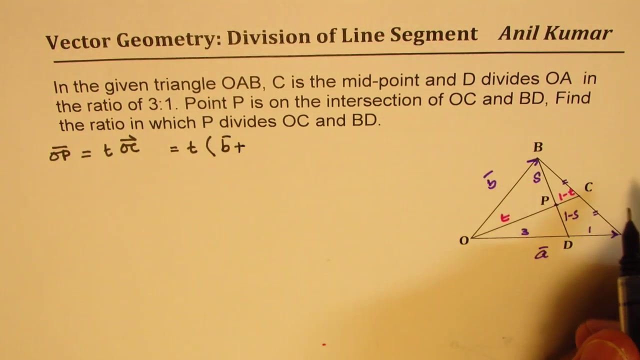 the vector OA as a vector. this, as vector B, should be easy. we write the answer in terms of a and B. so now what is OC? OC can be written as O to B plus B to C. so we have written vector B plus half of, because this is. 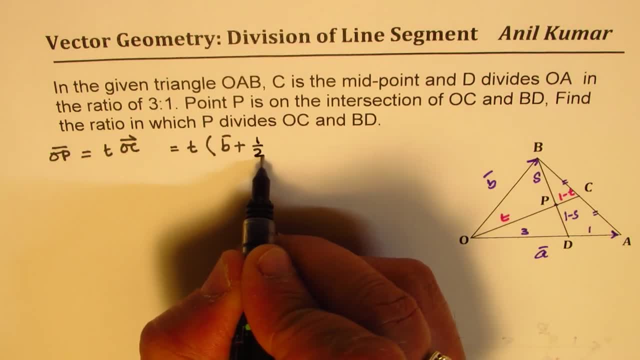 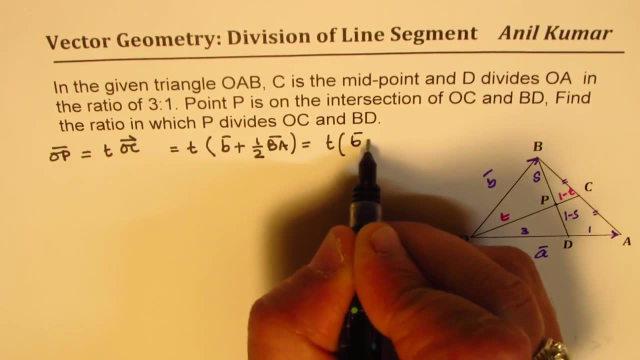 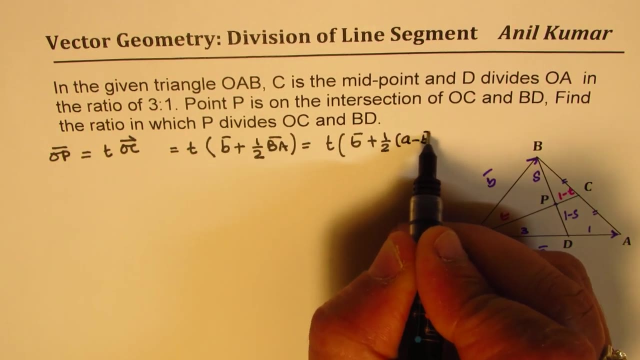 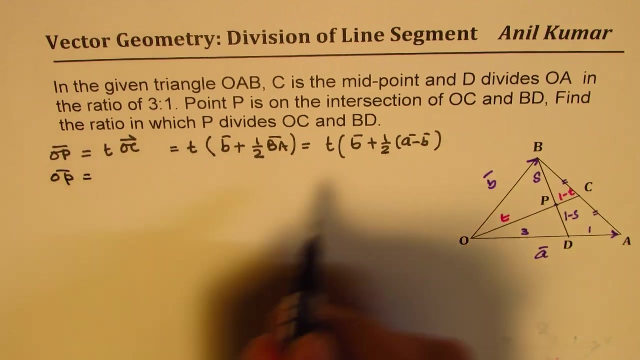 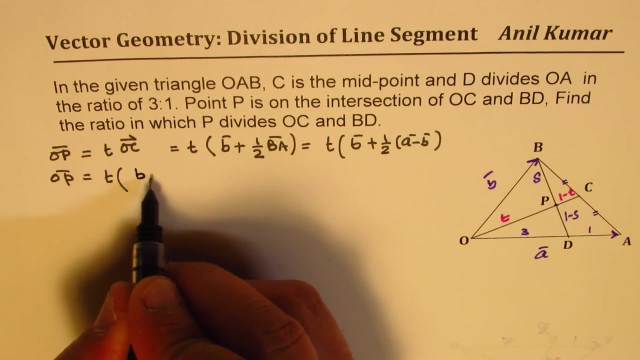 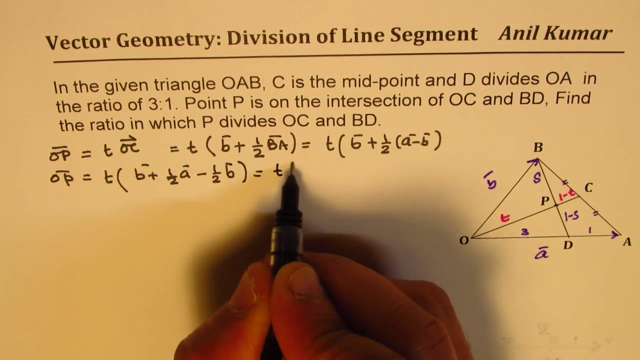 half of BA, right? so it is half of B to a. now what is B to A? b to a is a minus b, correct? So we will just open this. So we get op as basically equal to t times. So if you open this up, you get b plus half a minus half b or t times. 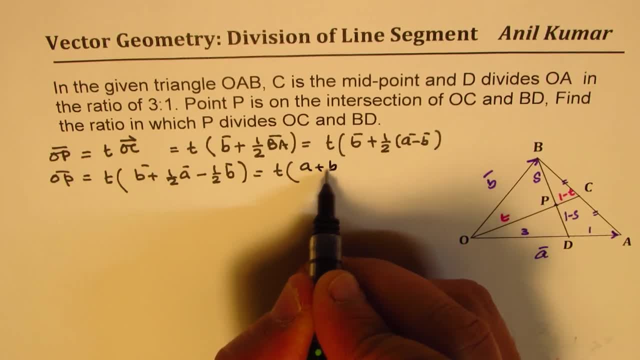 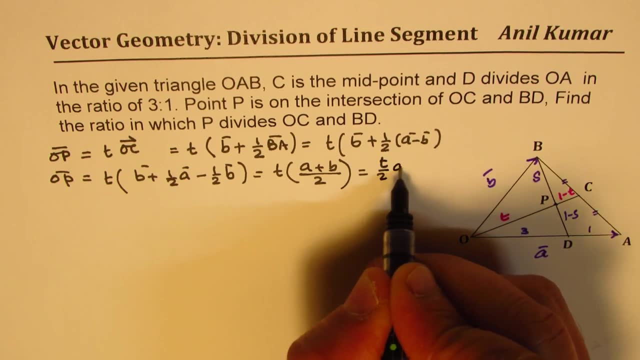 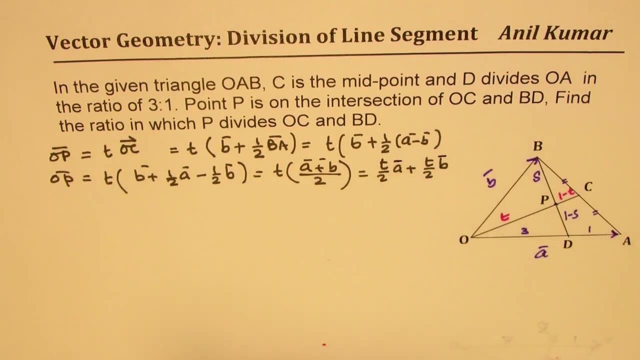 a plus b by 2, right, So we get a plus b by 2.. So I could write this as t over 2, a plus t over 2 b, right in terms of vectors a and b. So we got one of our equation. We. 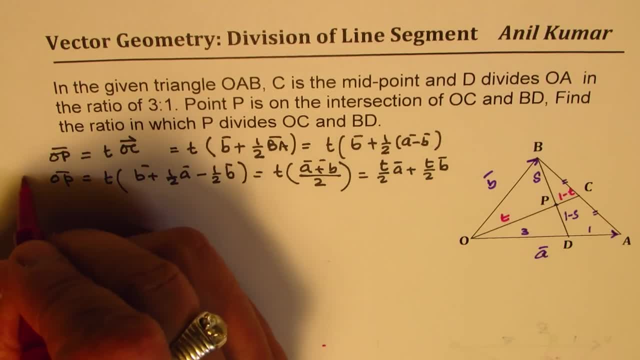 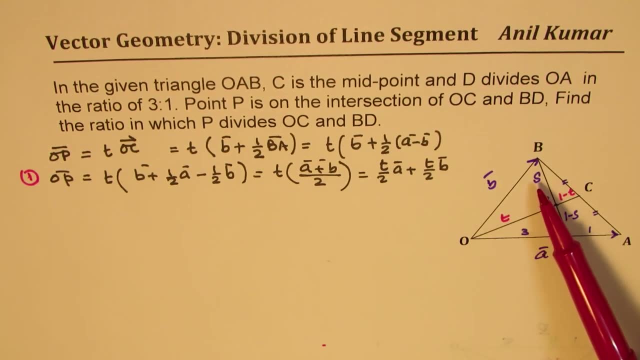 will call this as our equation number 1.. Let me write here: Now let us try to write op as a combination of a and b. Now, let us try to write op as a combination of a and b. So let us try to write op as a combination of this parameter s. So we could write op as: 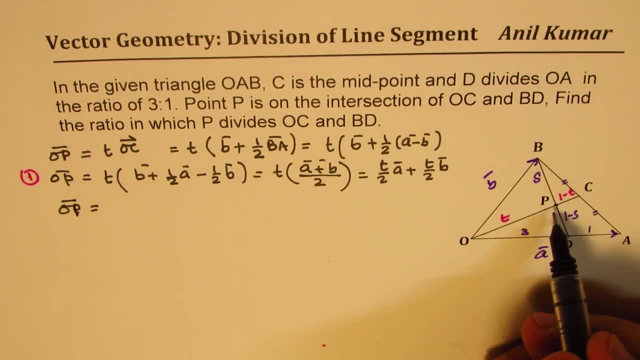 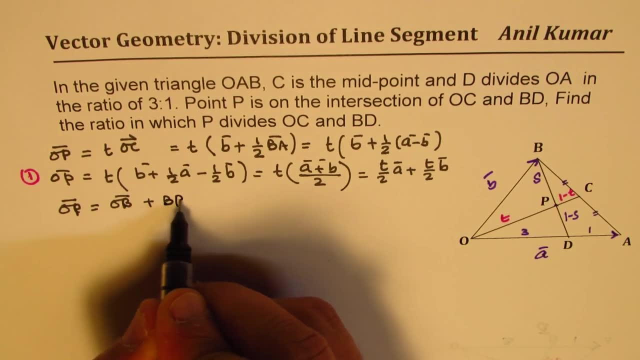 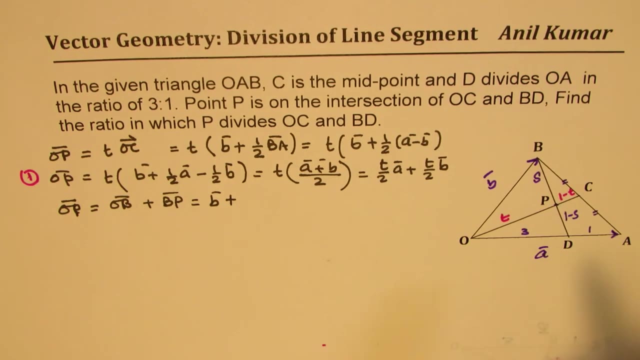 equal to. So we could say ob plus bp. So we say ob plus bp, ob is vector b plus b to p. Now how do we write b to p? Now b to p is s times bd, s times bd, So we can write. 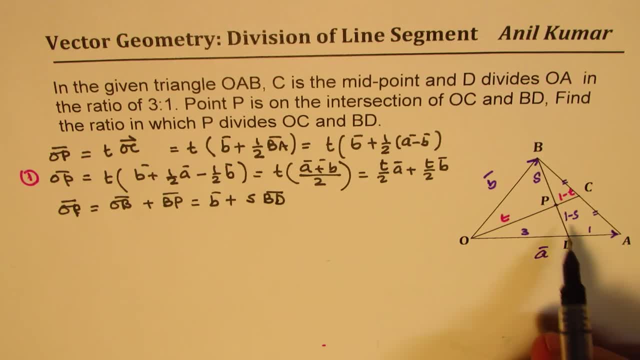 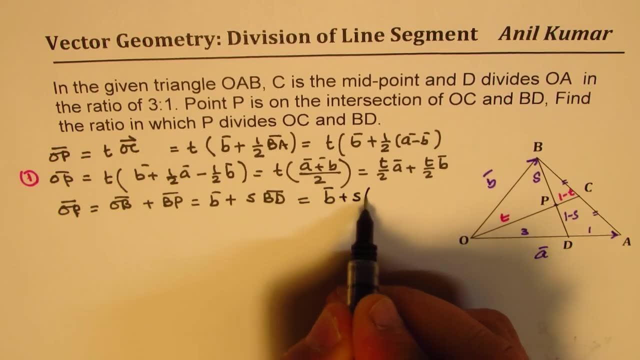 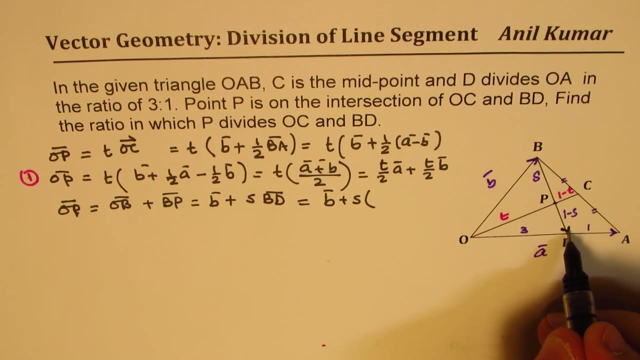 bd. What is bd? bd will be od right, So bd will be what? So? b times plus s times, What is bd? So b to d is So we want to go b to d, So we will come back here So. 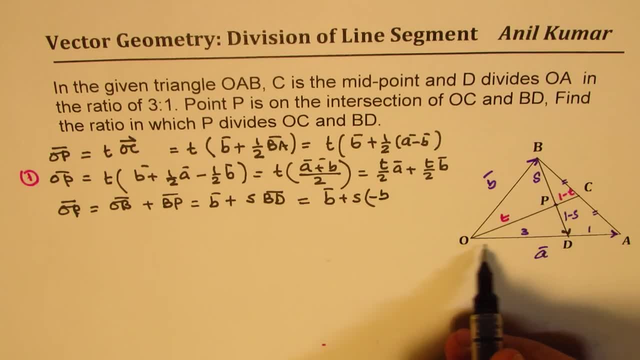 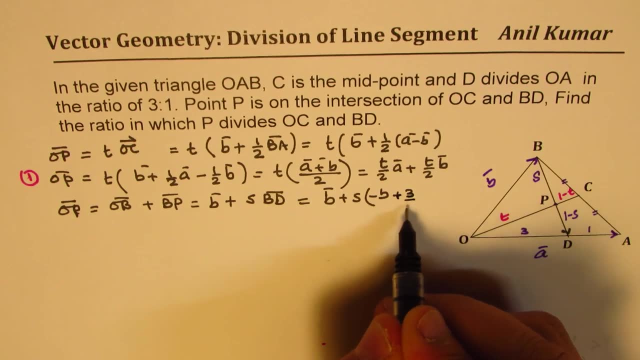 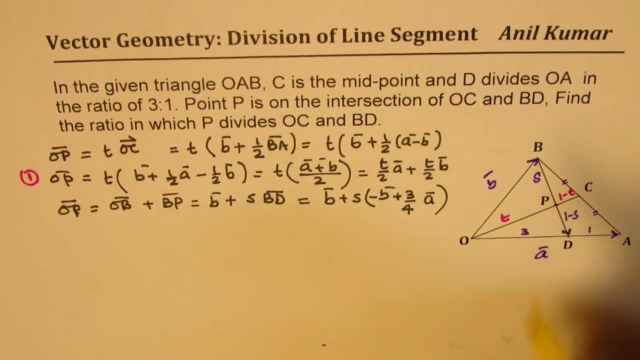 minus b right. We go in this direction and then there, which is 3 times a, 3 over 4 times a right plus 3.. Does it make sense to you? So what we did here was something like this: We want what? 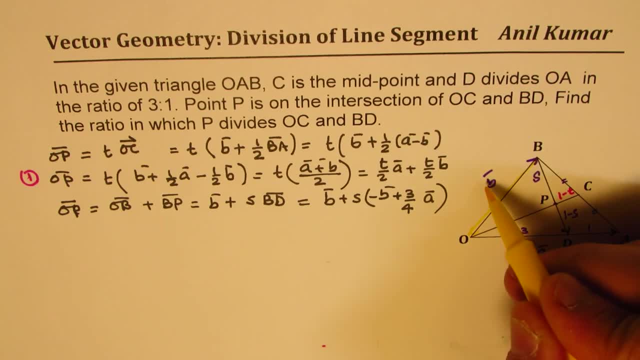 is b to d. So we came here, So this is a negative direction, negative b, and then went like this right. So 3 over 4.. This is total, is 4 parts, 3 plus 1.. This is 3 parts of a. 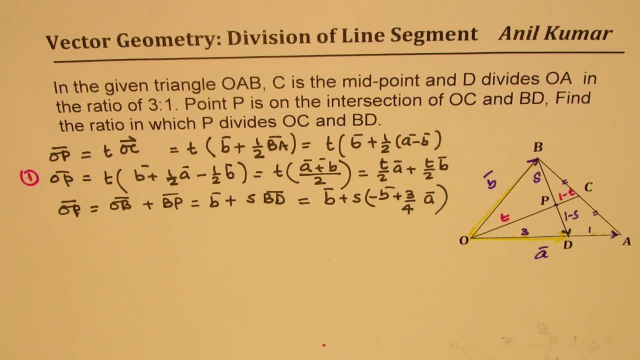 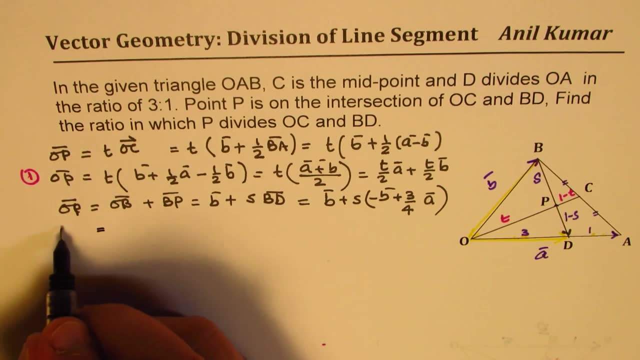 right. So that is how we get our equation. Now let us simplify this one and isolate it a and b, just as we did that, So we can now write op as s times 3 over 4 a, So we can. 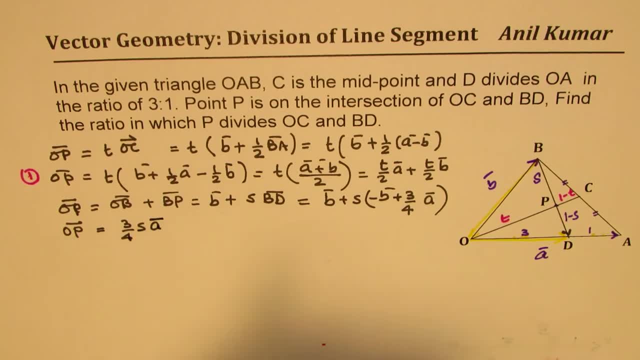 write 3 over 4 s times vector a. As far as b is concerned, we can take b common 1 minus s, right 1 minus s, So that is how we can write this vector. So we will call this as. 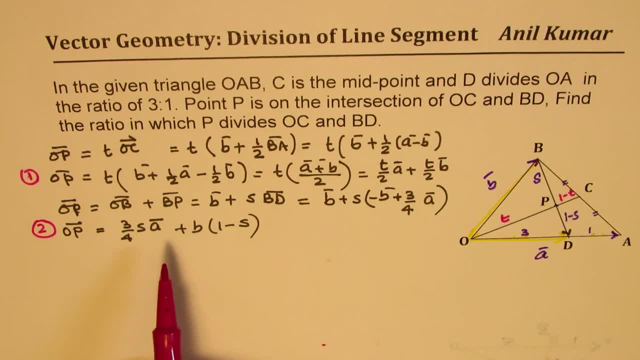 our equation number 2.. Is that clear? So what we did was We actually found two different ways of defining op right, And in doing so we have involved both t and s, the two parameters in which we are really interested in. Now, how do we? 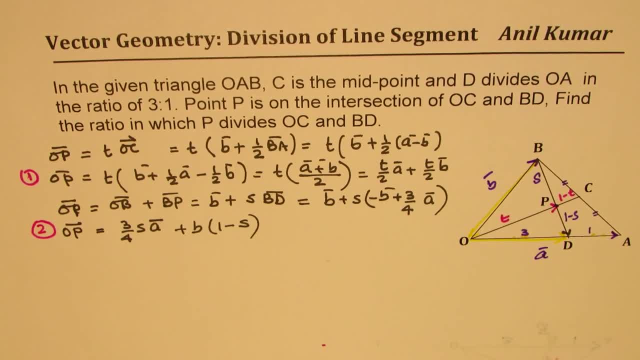 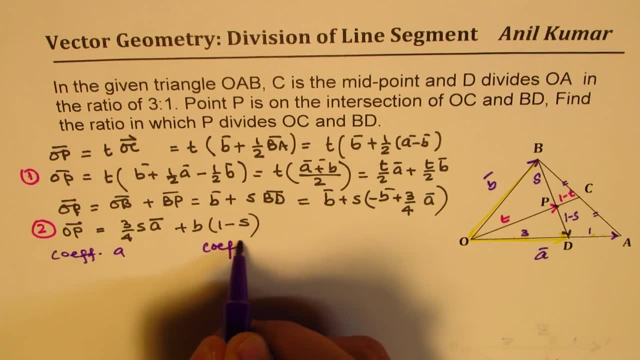 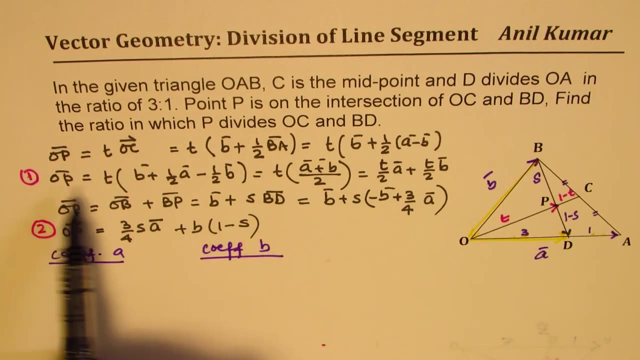 get their values. So we get it by comparing right. So coefficients of a and coefficients of b, We compare these two coefficients. Now we can take our coefficients to get our equations and we will solve them. So in equation 1, the coefficient of a is t by 2.. So we get t by 2 should be equal to in: 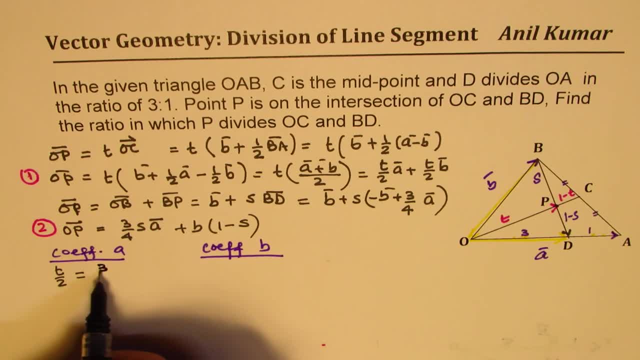 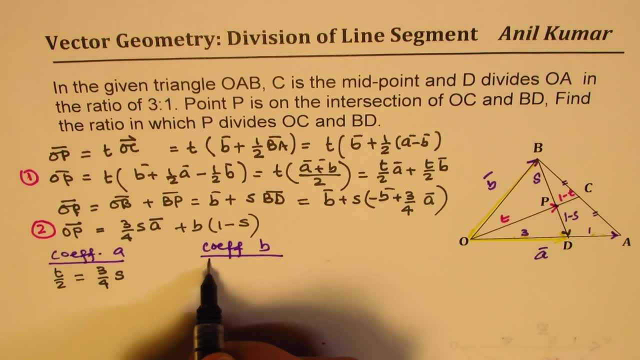 equation 2, it is 3 over 4 s. In for coefficients of b. it is t by 2 for b and here it is 1 minus s. You see that. So we get our coefficients right Now. we can store them here. We do not. 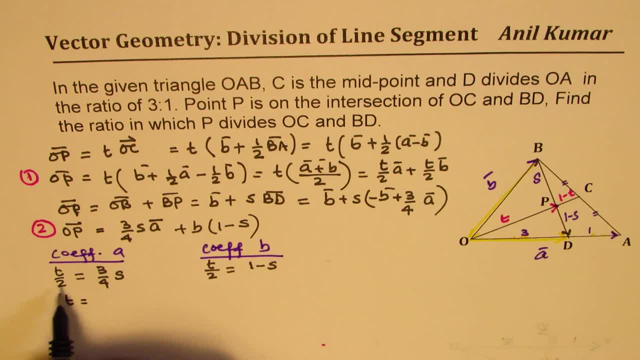 have to do it again. So we will do it again. So we will just write our coefficients. So that is how we get our coefficients. Now let us take our coefficients right. Now. we can solve this. we get T equals to when you multiply 6 over 4, or rather 3 over 2s. 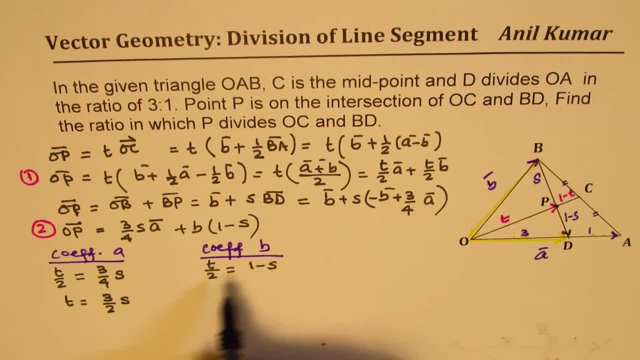 now, here we know what s is in terms of T, or either way, we could write s here, right so, or we could eliminate, right so. what we will do here is basically: T is equals to 2 minus 2s, so replace this value of T with 2 minus 2. so it was. 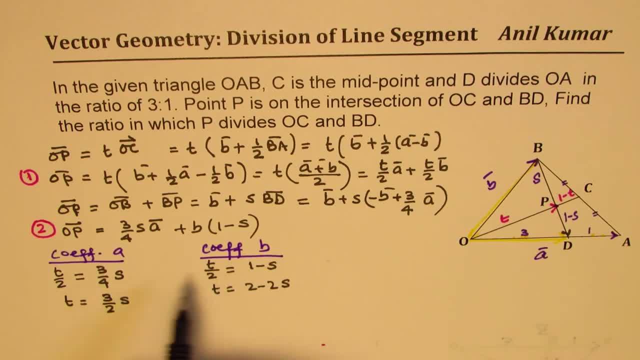 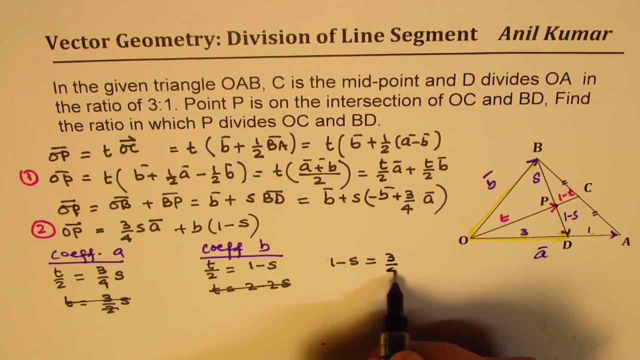 better to use T by 2 itself. we could have written 1 over s, right, so so we'll just forget about this. we have t over 2 s, 1 minus s and t over 2 s, 3 over 4 s. that means that means that 1 minus s should be equal to 3 over 4 s. clear right. 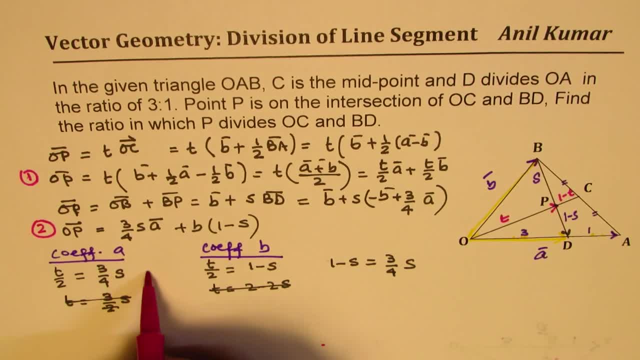 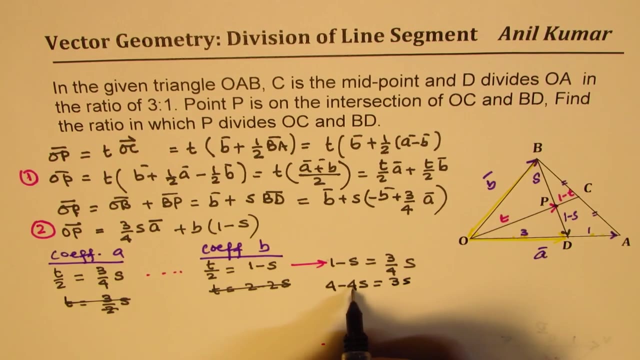 so from here itself we can actually get better our equation right. we get this: t over 2 is 3 over 4s and 1 minus, so they are equal. okay, this is better. so now we'll cross multiply so we get 4 minus 4s equals to 3s. taking it on this side, we 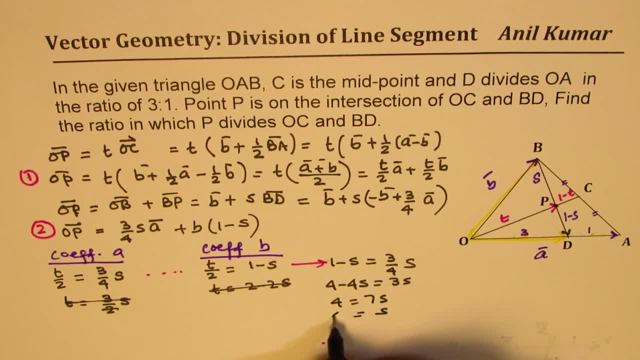 get 4 equals to 7s, or s is equals to 4 over 7, so we get the value of s. now from here we can get the value of t. so t is 3 over 2s, which is 3 over 2 of 4 over 7, 4 over 7, right? so s is 4 over 7, so we 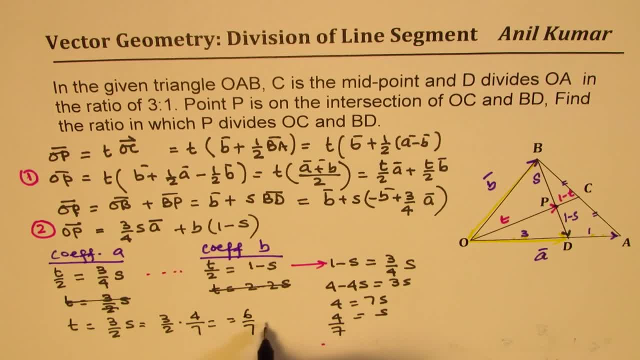 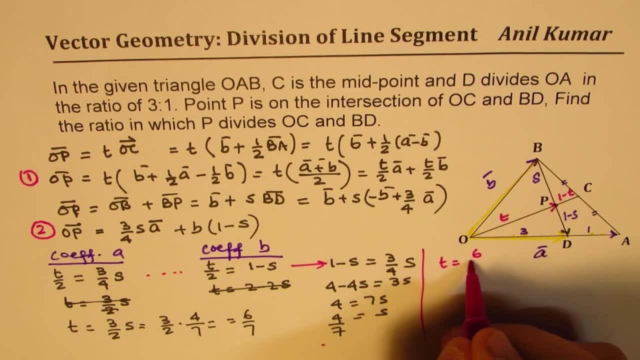 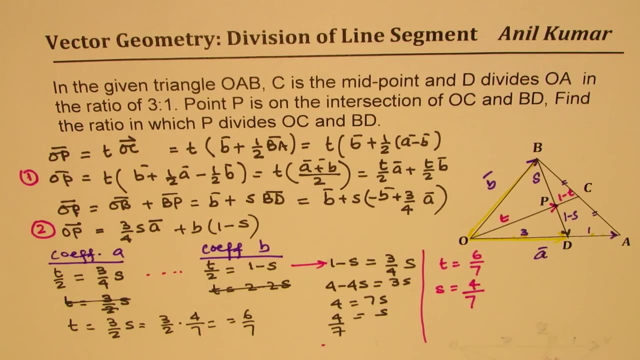 get here. that goes: two times 6 over 7 is a value of t, right? so we got both the parameters. so you are saying t is basically equals to 6 over 7 and s is equals to 4 over 7. so right, so so this is cancers two times 6 over 7. and here we get 4 over 7. that's correct, so that 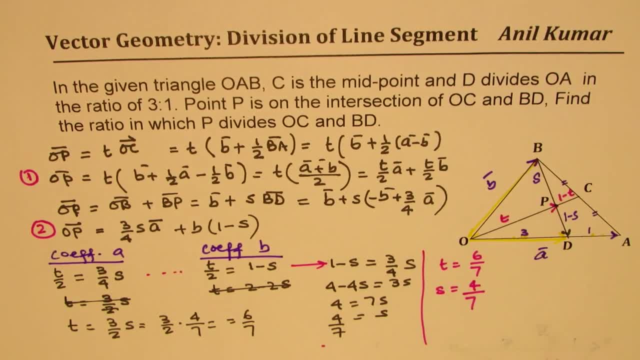 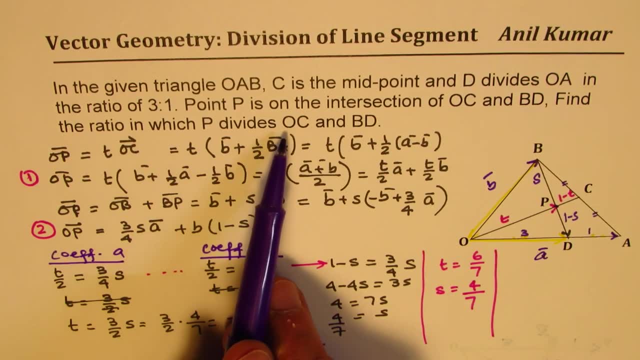 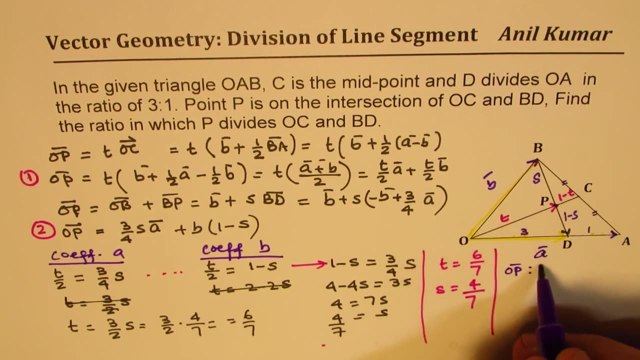 is how we get our parameter s and t, and now we can write down our answer right. so we want to know in what ratio p divides oc and bd. so as far as oc is concerned, we can write: the ratio op is to pc is what? since t is 6 over 7, that means total divisions are 7. so it is 6 is to 1. you get the. 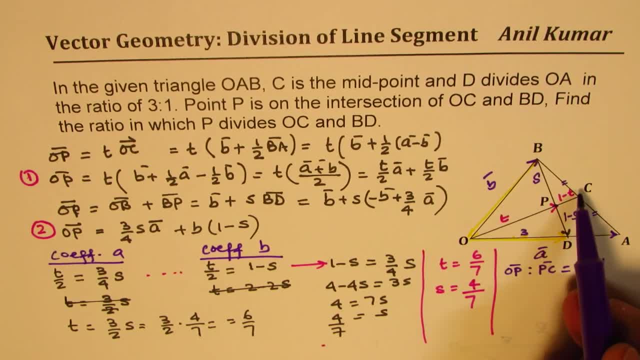 idea 6 over 7. so total is: this is 1 out of 7. this is 6 out of 7. as far as bd is concerned, the ratio of bp to pd is what s is: 4 over 7. so 4 here, 3 there, 4 is to 3. 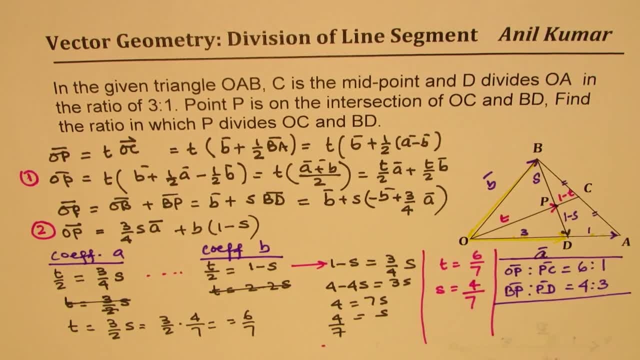 over 5. so 4 is equal to 4 over 7. root over 5. there is 0, 0, sorry, 4. 3. 1 over 7. this is 4. there is 1 and 7 here, right, so it is 7 over 7. so we want to know x to the power over 7, right plus x to. 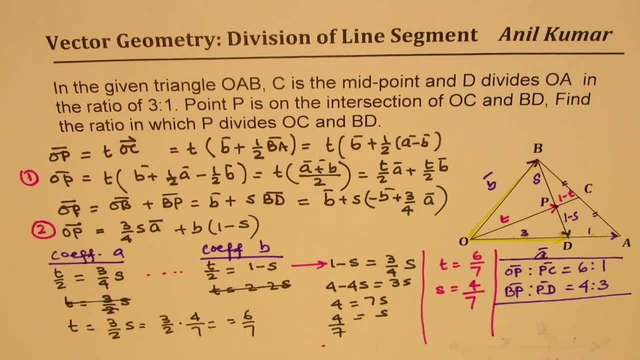 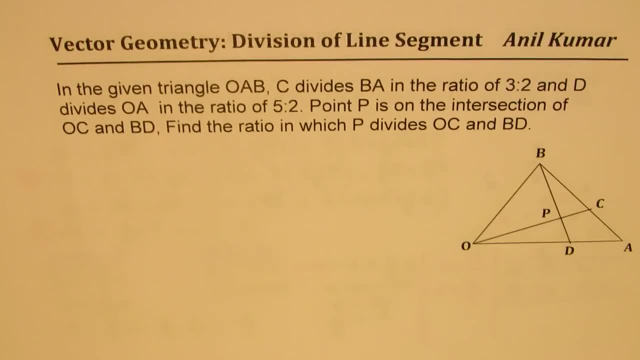 the power of 3 and 5 plus 2, we can set 7 over 7. so the answer is ok. but now we just go to the other thing. the answer is equal to 2. so what we just wanted to explain is that, perhaps, since we want to know how this sum is going to change our class here, our size, whatever, 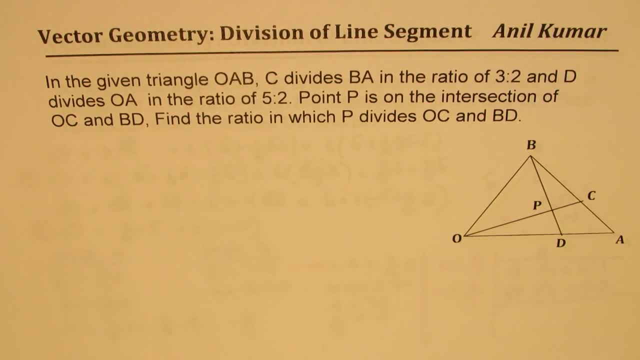 way that we areSu q is equal to 10 for ourFe? eld videos including. this is our original class, and since this question is difficult for me now, i'm going to give you a test so and post your answers in the comments. I'll provide you the solution of this. 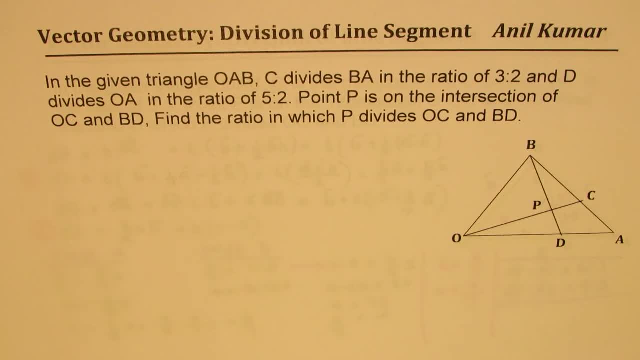 question later. I hope you understand and appreciate how we have solved these questions. Feel free to write your comment, share your views and, if you like, and subscribe to my videos. that'd be great. Thanks for watching and all the best.